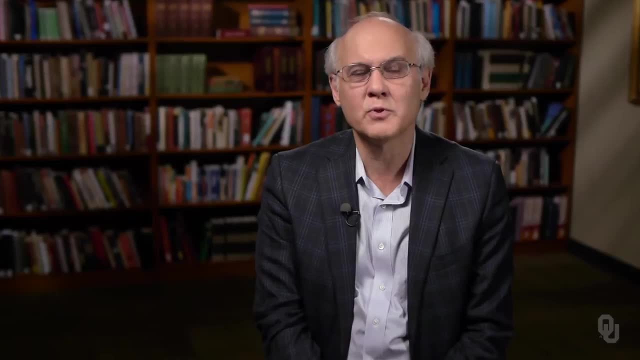 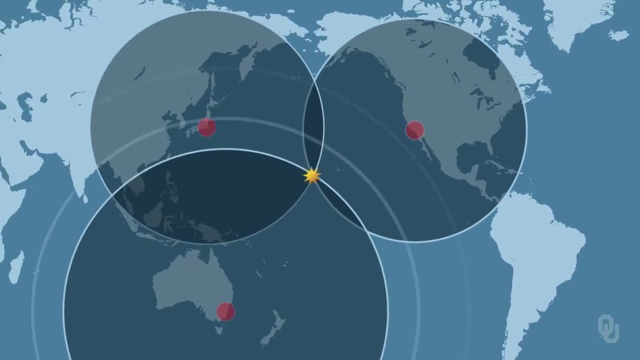 how far you are from a quake based on the time difference between the P and the S wave, Then you need three seismograph stations to triangulate and locate the earthquake epicenter. I would like you to learn about earthquake waves and how they can provide information. 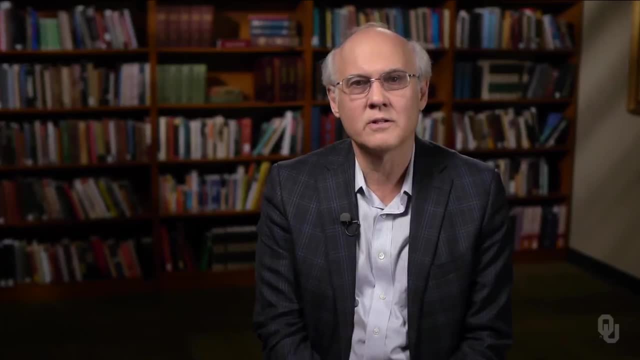 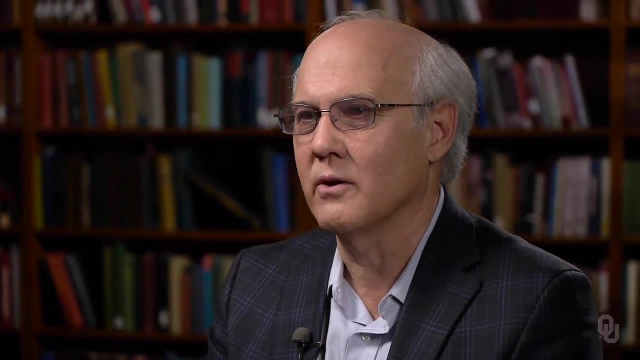 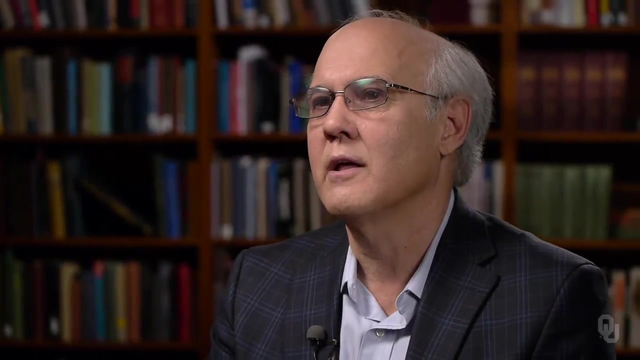 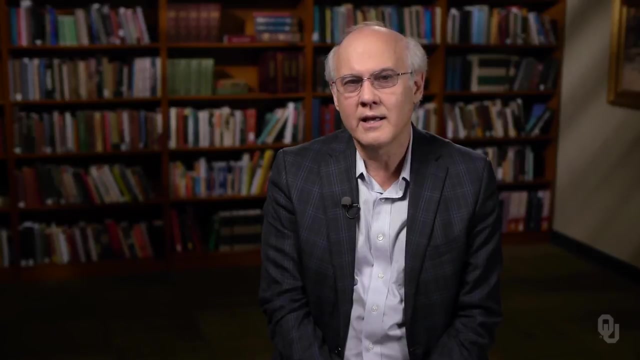 on the structure of the earth by examining your class notes and the textbook that we have online. We'll now talk about earthquake intensity and magnitude scales. There are two scales that you commonly see when we talk about earthquakes and the severity of those earthquakes. The first is the Richter scale and it measures the energy released. It's a scale from 1 to 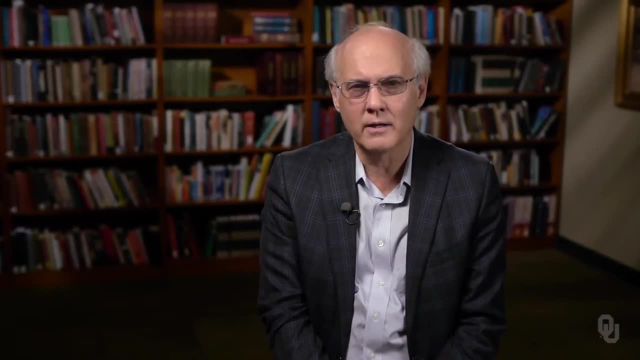 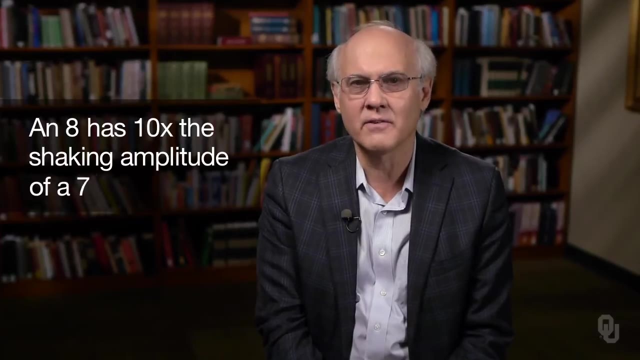 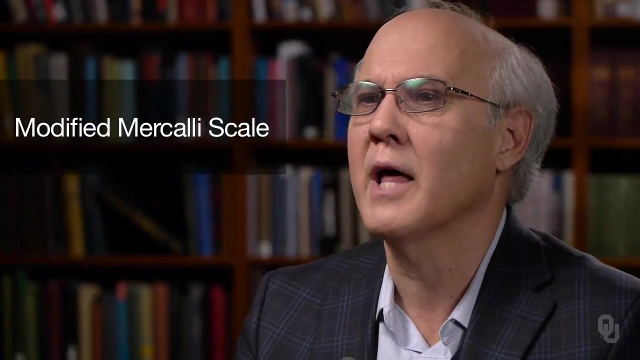 10, and 8 is a very big earthquake, And what's important is that an 8 on the Richter scale is 10 times as strong as a 7 on the Richter scale. Another scale is the modified Mercalli scale and it measures how people and buildings are. 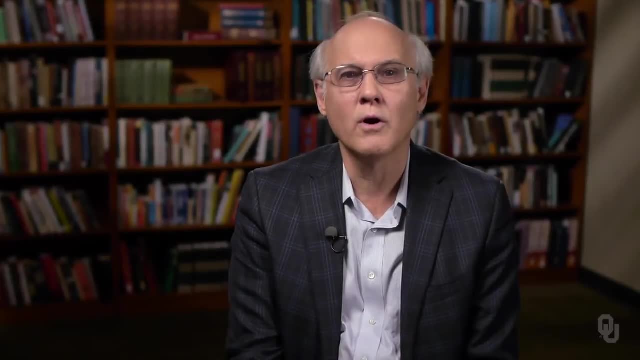 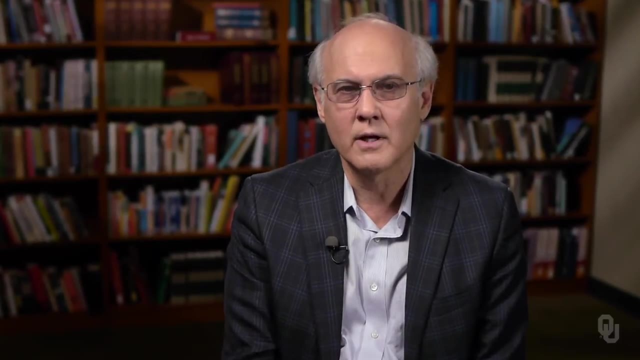 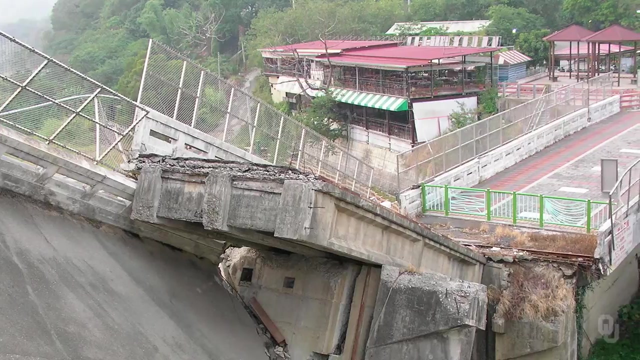 affected by earthquakes. For example, a 4 on this scale is that most people will feel it indoors and dishes, windows and doors will rattle. A 10 on this scale is most buildings and their foundations are destroyed. Some bridges are destroyed, So it's based on how. 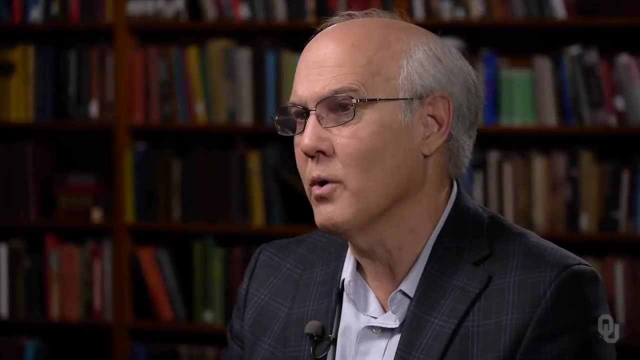 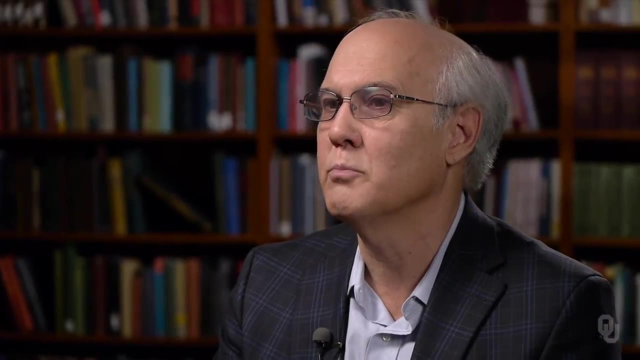 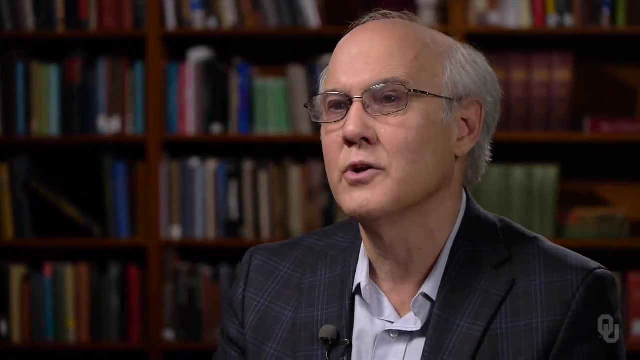 it affects us and buildings. Another important topic with earthquakes is prediction of quakes, And I'll start off by saying there is no foolproof way to predict when an earthquake is going to occur. There are various methods that have been used in the past to predict earthquakes, For example: 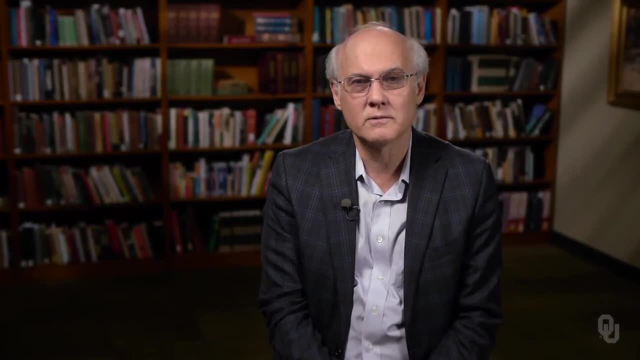 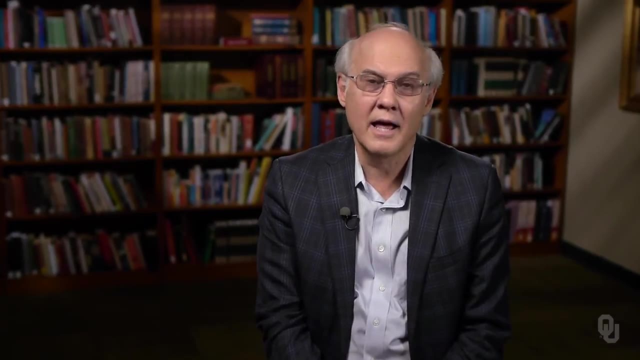 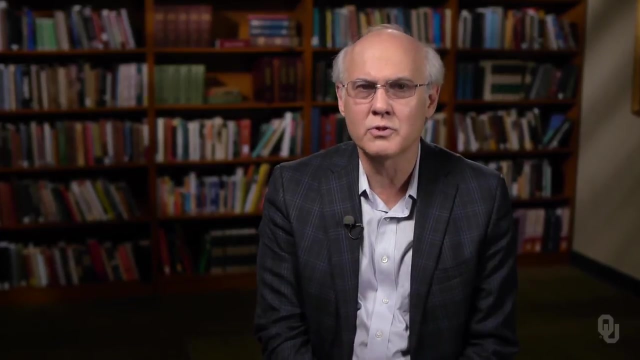 in China. they used the behavior of animals. In some cases they would have been able to predict large earthquakes. In other cases they were not and thousands to hundreds of thousands of people died. Subtitles by the Amaraorg community. Other kinds of things you can look at to predict earthquakes or use to predict earthquakes include: 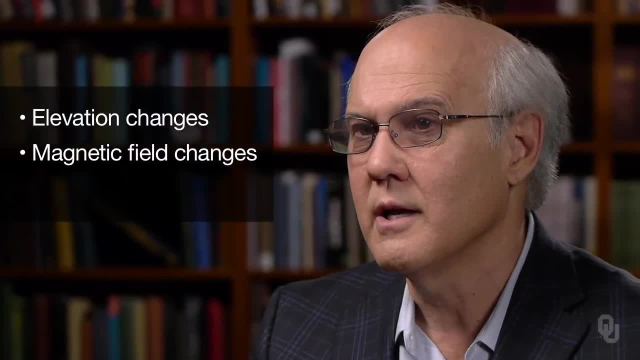 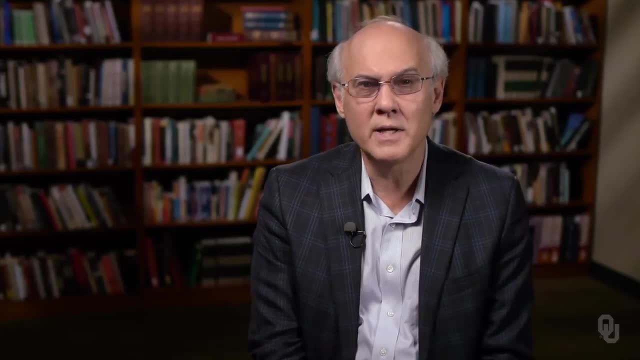 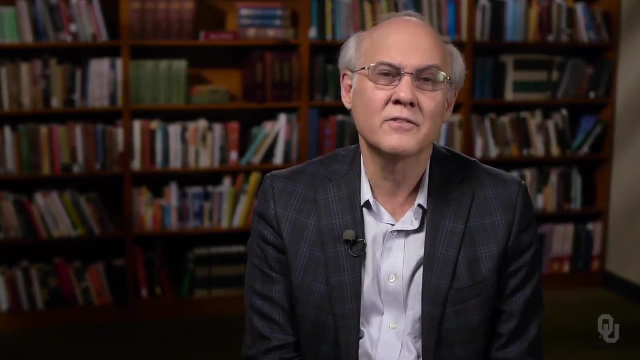 elevation changes, magnetic field changes and seismic gap ideas. The idea of a seismic gap is the following: If there is a recent quake along one segment, then stress has been relieved along that segment. So it is not likely there will be another quake in the near future. If there has not been a recent quake and stress is building,